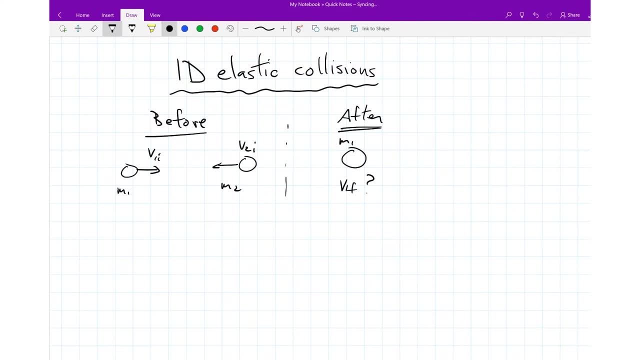 an object with mass m2 moving to the left with initial velocity v2i And after. my goal is to find what are the final velocities of m1 and m2.. So we start off with momentum conservation and since this is an elastic collision, we also have conservation of kinetic energy. 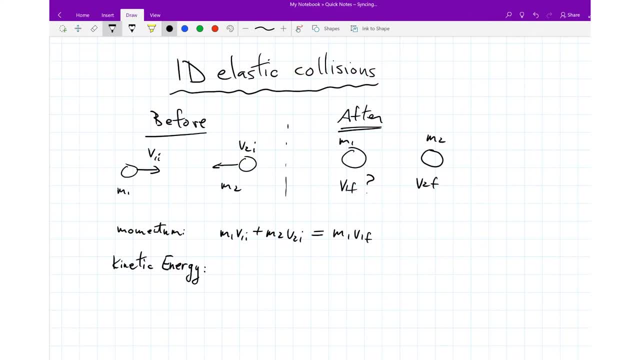 For momentum, simply write m1 multiplied times v1 initial, plus m2 times v2 initial, and that has to be equal to the final momentum after the collision. For kinetic energy, it's pretty straight forward: You simply write the kinetic energy of each object before and. 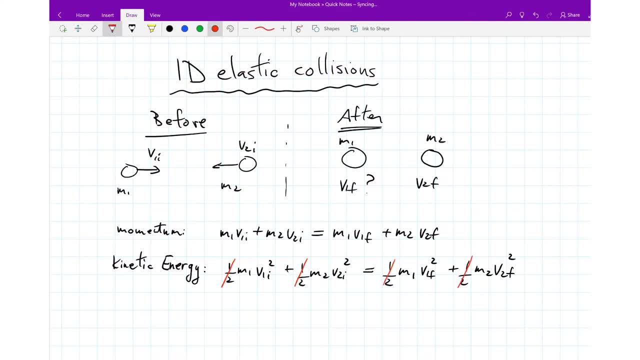 after the collision. You can simplify the one-halves and the kinetic energy, since they appear in all the terms, And we can also simplify the expression by grouping all the terms for object 1 on the left-hand side and all the terms for object 2 on the right-hand side. 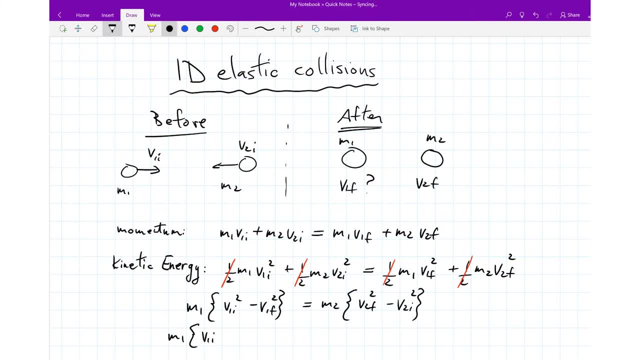 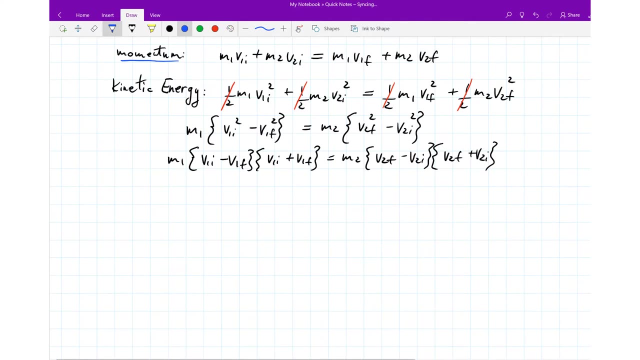 Now, this is a difference of squares. This can be simplified, So, for each side, we simply can break that down into two parts, One that has a negative sign and one that has a positive sign, And at the end we're left with this final expression. 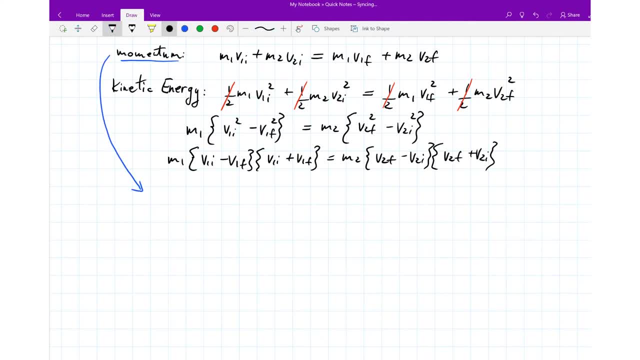 Next let's work on our momentum equation. Again, we're going to group all the terms with object 1 on the left-hand side of the equation and all the terms with object 2 on the right-hand side. So on the left-hand side we're going to have initial and final velocities. 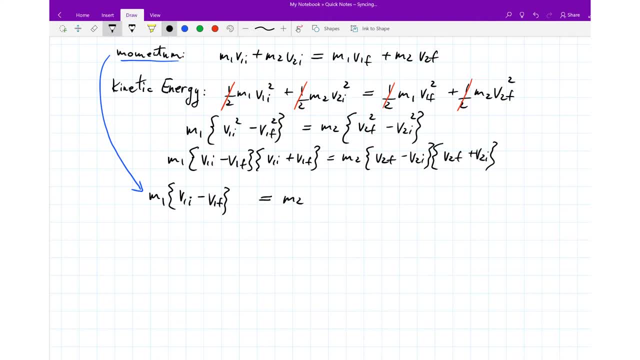 end up being the difference between the two, And for object 2,, again you're going to have the difference. The final and the initial subscripts end up being reversed. but that's okay. It's just how the algebra works out. 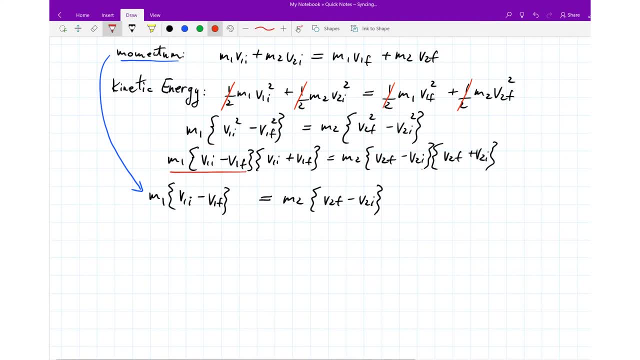 The next thing to realize is that this momentum equation is exactly the same terms that appear in our kinetic energy conservation equation. So we can actually simplify the kinetic energy expression by canceling out both of those terms. And if you simply just rewrite it now: 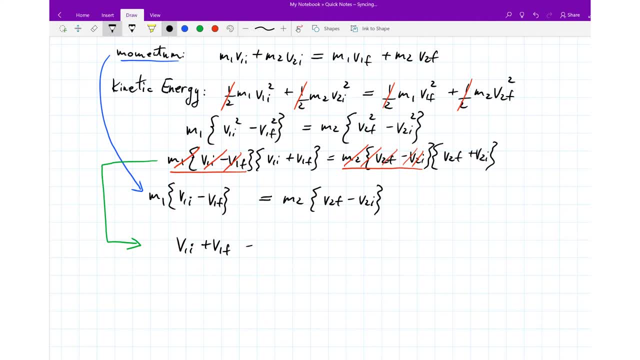 and not including the eliminated terms. you simply have: the initial velocity plus the final velocity of object 1 equals the final velocity of object 2. And that's the final plus the initial velocity of object 2.. This really greatly simplifies our expression for the kinetic energy. Now to take things. 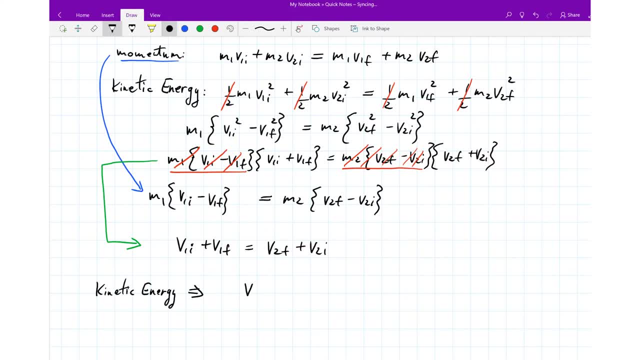 even one step further. I'm going to group all of the initial velocity terms on one side of the equation, So you bring v2i on the other side and you group all the final terms on the right-hand side. In order to keep the same form, I'll just factor out a negative. 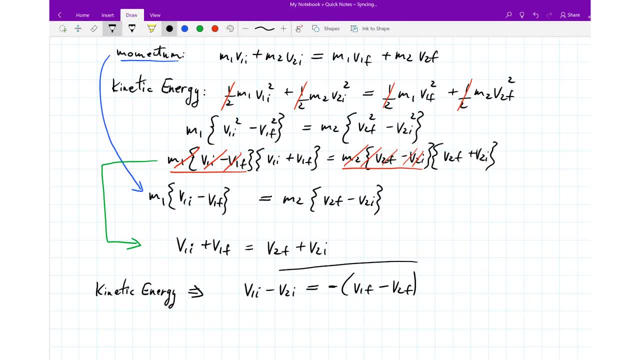 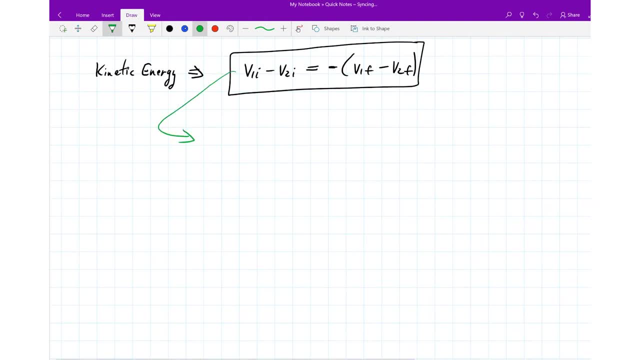 sign And, at the end, our kinetic energy expression boils down to this simple expression. So what does this expression actually mean? This expression simply means, if I just look at the left-hand side, v1i minus v2i. this is simply the relative velocity of object. 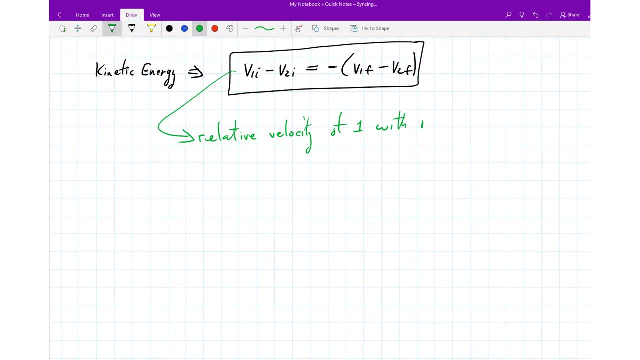 1 with respect to object 2.. And we're looking at the initial case before the collision And the right-hand side is simply the relative velocity. again after the collision, There is a negative sign that pops up there, but that's okay. 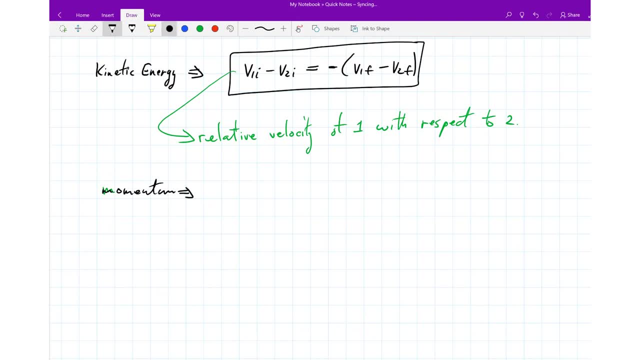 So let's just simply rewrite our momentum equation once again, because we still have two equations and two unknowns. Our momentum equation- that was one of the first equations we wrote down. That was simply the sum of the individual momentums before and after. 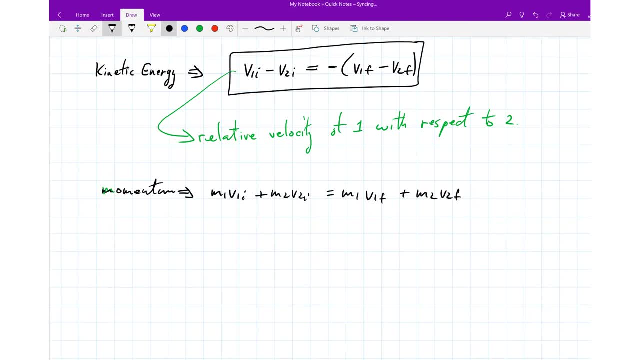 the collisions of each particle. And now the system of equations is simplified. The momentum equation is our equation 1, and the relative velocity equation, which is this kinetic energy equation, is v1i And the equation 2 is equation 2.. Now let's take equation 2 and multiply it by m1 on both. 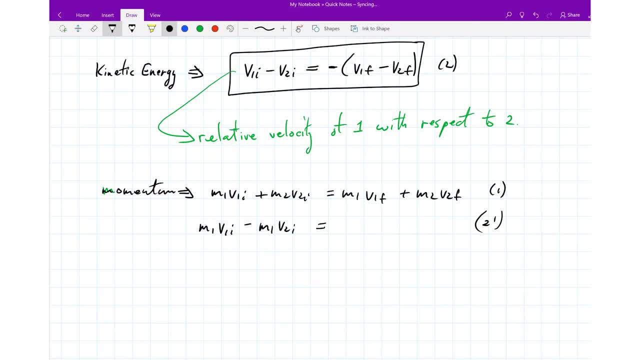 sides of that equation and rewrite it. This is what it looks like. Again, you're simply multiplying m1, and I factored out the negative sign on the right-hand side of the equation. The reason I do this is because I want to simplify the equations I want to end up getting. 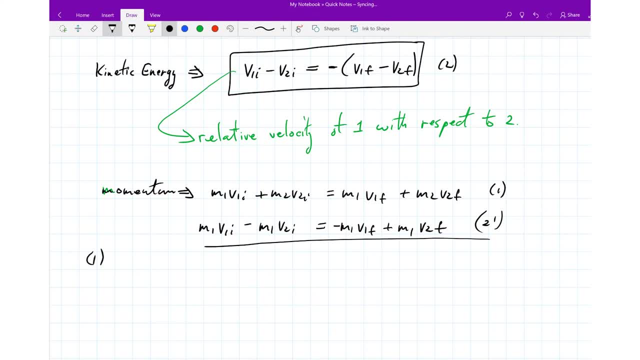 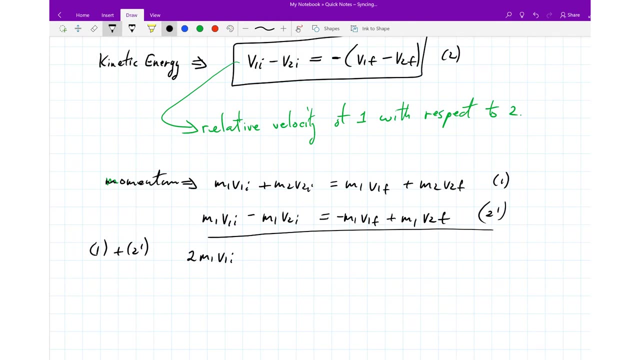 an expression for v2, final. And if I multiply by m1, now I get a slightly modified equation At the end. if I add equation 1 to equation 2, prime, I'm going to get this following expression: – 2m1 v1, initial, The terms with: – oh, those don't cancel One second I'll have. 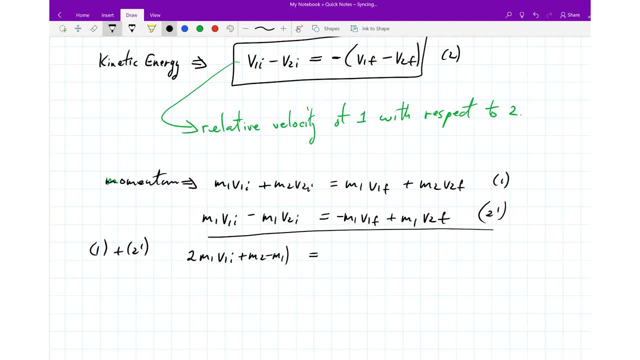 to add those in here. You still have a combination here with m2 minus m1.. That multiplies the initial velocity 2.. Now the next term will cancel out And I'm only left with – the right-hand side has a term that multiplies the final velocity. 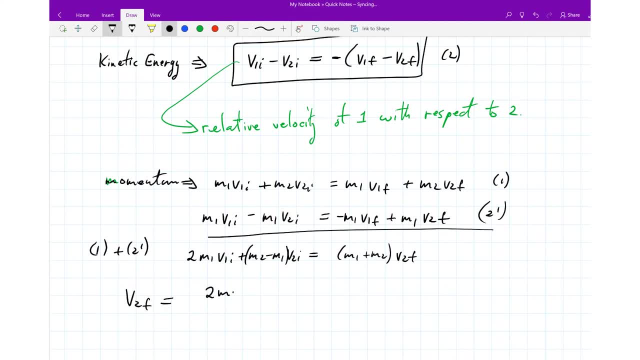 of object 2.. So if you divide through by the total mass, m1 plus m2, you're going to get one final expression for the final velocity of object 2.. And it looks something like this: There are two contributions. There's a factor that multiplies the initial velocity of object. 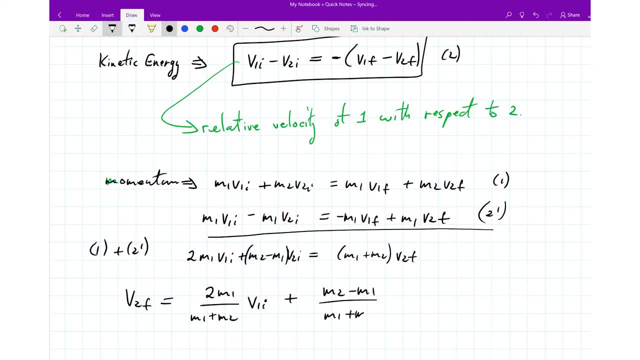 1, and there's going to be a slightly different factor involving the masses of both objects that multiplies the initial velocity of object 2.. And I'm only left with – the right-hand side has a term that multiplies the final velocity of object 2.. So if you divide through by the 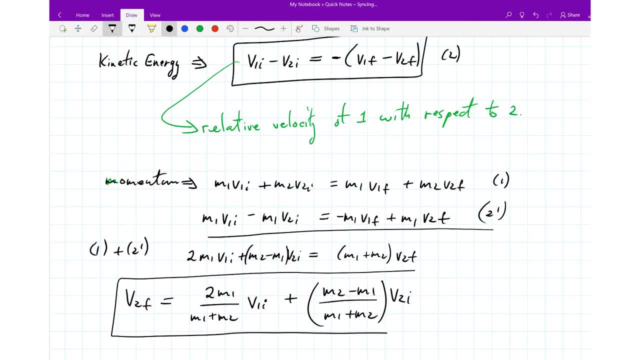 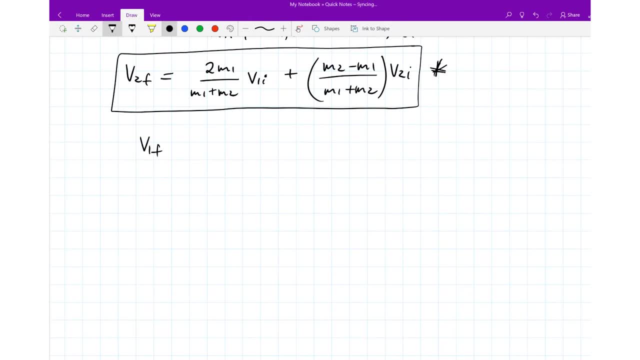 object 2.. And that's it. So I have now a final expression for the final velocity of object 2.. To find the final velocity of object 1, I'm going to use the modified kinetic energy equation, which was the one dealing with relative velocities between the two objects before and after the 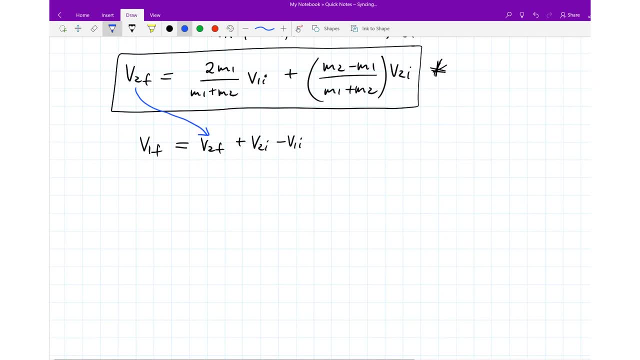 collision, If I rewrite it slightly differently. and now all I have to do is substitute the expression I just got for object 2 into this equation. So you've got to substitute both terms in there. After we're going to have to do a little. 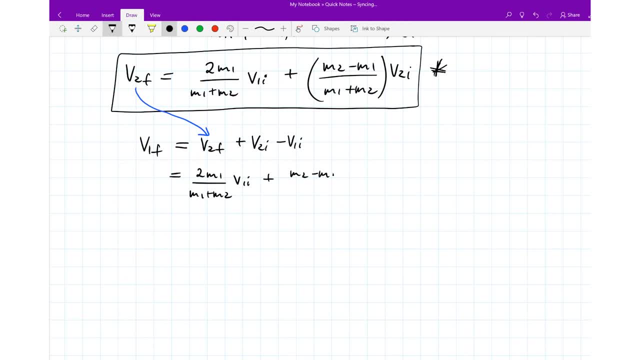 bit of algebra in order to group together the factors in front of the initial velocity for object 1 and the initial velocity for object 2.. But if you do a little bit of math, you should end up with a similar expression to what we got for object 2.. 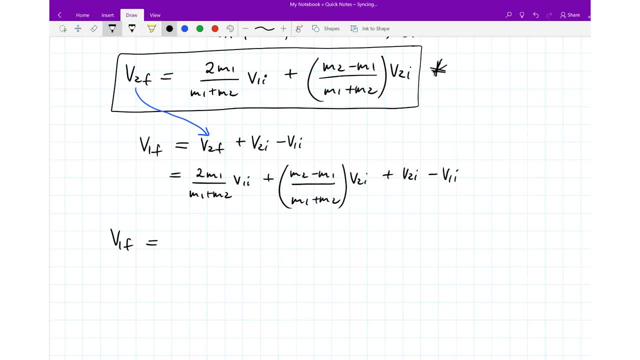 So again, we're just going to carry out the algebra now. You see, the first term and the final term involve the initial velocity of object 1.. We can group those. And the two middle terms involve the velocity of object 2, the initial velocity of object 2.. So again, if 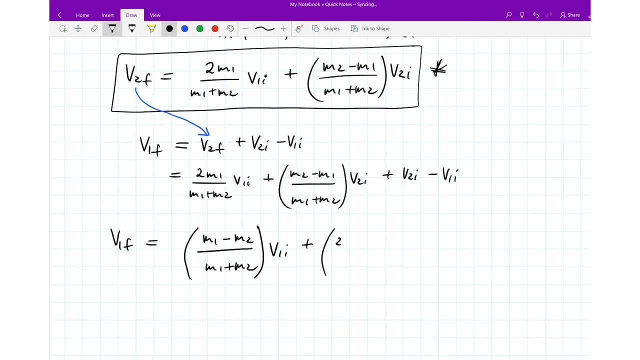 you group everything together. this is the final expression that we get for the final velocity of object 1 after the collision. It involves the same factors or similar factors. There's negative signs that kind of end up coming in there and that's okay. 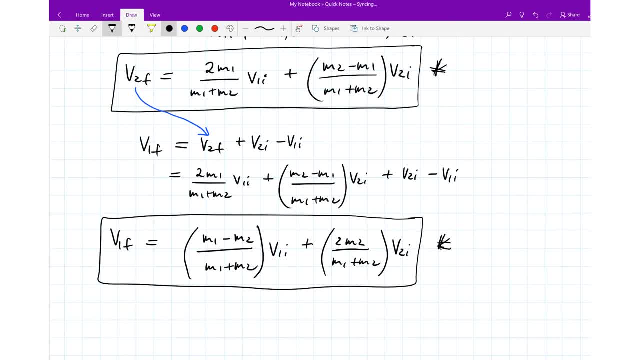 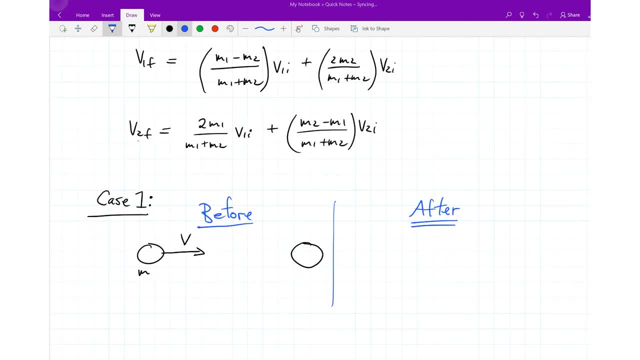 We're going to apply these equations in just a moment. All right, so I now have two expressions: one for the final velocity of object 1 after the collision and 1 for the final velocity of object 2 after the collision. I want to consider now four different collisions. This is case. 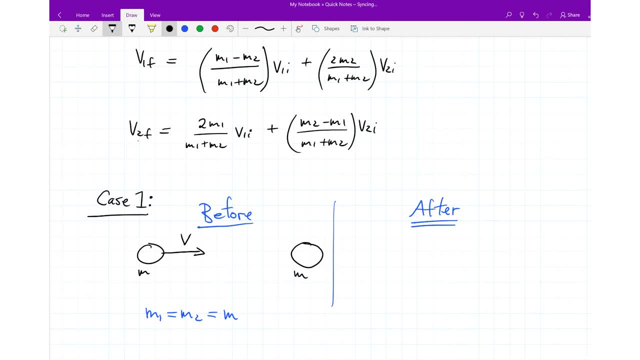 one that I've drawn here on the board. We're going to consider the mass of the, the objects, to be the same, and we're going to have object 1 that is moving to the right and object 2 that's stationary, so it has no initial velocity. I now want: 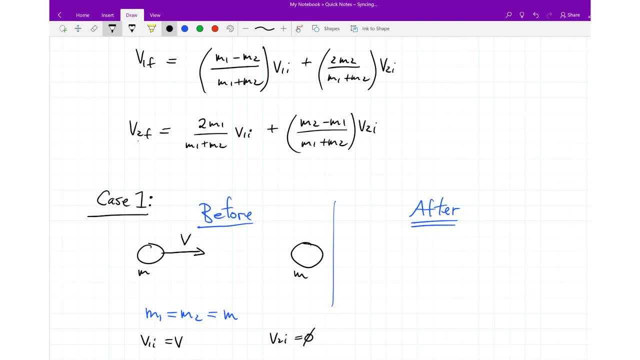 to set up the equations and find what are the final velocities of object 1 and object 2 after the collision. So again, they both have the same mass. so that'll simplify some of the terms in our expressions above. The initial velocity of object 1 is V and the final velocity of object 1 can be obtained using the. 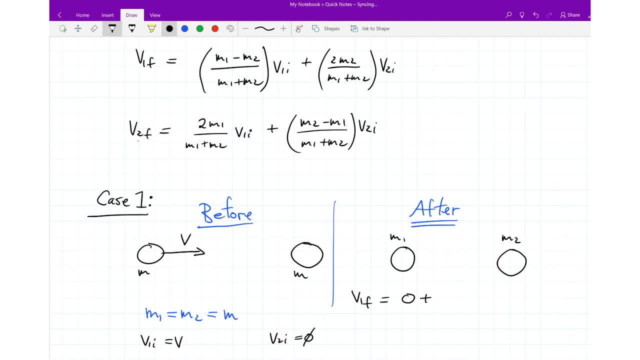 top equation. Since the masses are the same, the first term equals to 0 and the second term again. if you simplify it a little bit, since the initial velocity of object 2 is 0, you're going to get 0. The final velocity for object 2. now, if you 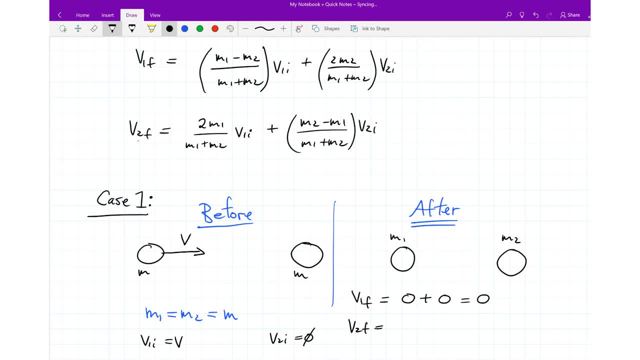 substitute in the numbers. again masses are the same, so that simplifies. So the first term simply becomes 2m divided by 2m. So the first term simply becomes 2m divided by 2m. So the first term simply becomes 2m divided by 2m. 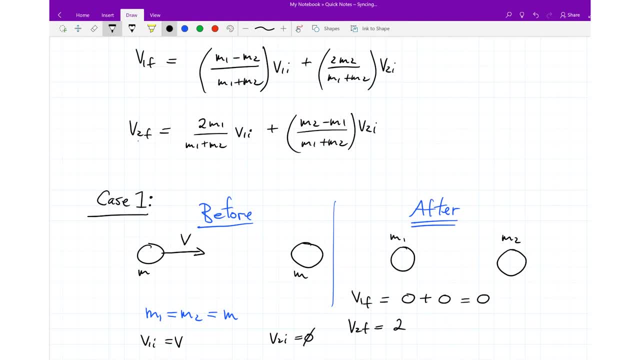 Since the masses are the same, multiplied by the initial velocity of object 1, which is simply V. So we're going to get 2m1, simply 2m, rather divided by 2m, for that first term, multiplied by V, The second term, since. 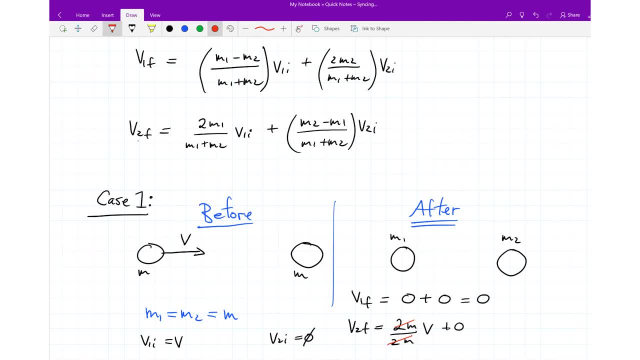 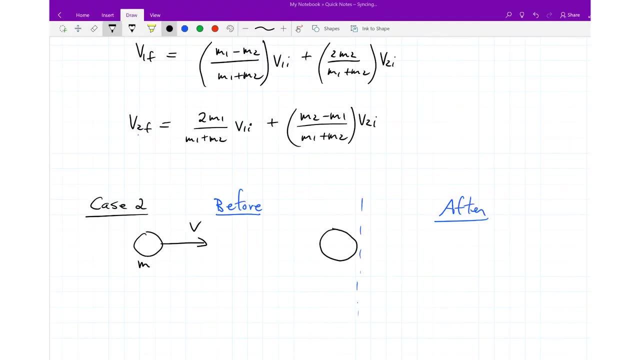 the masses are the same equals to 0. So the 2m's can cancel out and we're left with the final velocity of object 2 is simply V. Alright, so when we have a collision like this, object 2 is simply going to move to the right after the collision. for case number two now, I want: 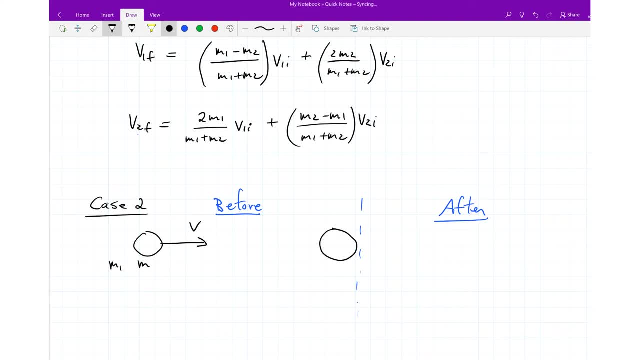 to take the limit where object 2 is much, much bigger than object 1. therefore, its mass is going to be much, much greater than object 1.. It's going to be stationary initially and object 1 is going to be moving toward it and there's 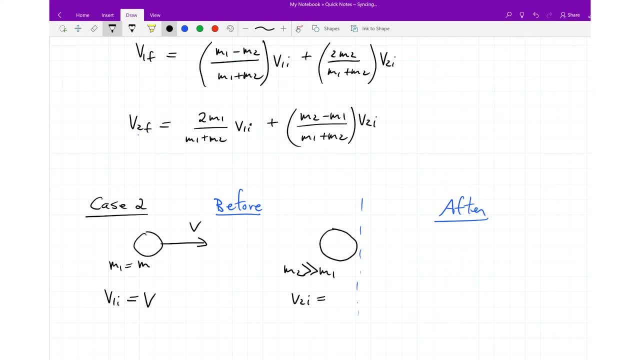 going to be a collision. Object 1 is moving at some velocity V and again, object 2 is initially stationary and object 2 is moving at some velocity V. Now, if you take the limit when m2 is much, much bigger than m1, you basically 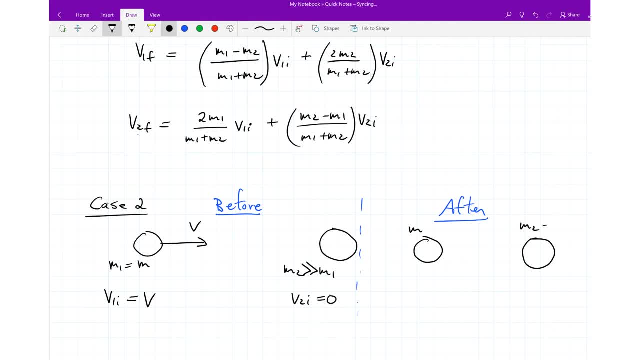 don't have to consider the mass m1 in our expressions above, so it simplifies a lot of the terms. So what happens after the collision? Try it out for yourself. So again, you don't have to consider the impact of m1 anymore, because m2 is a. 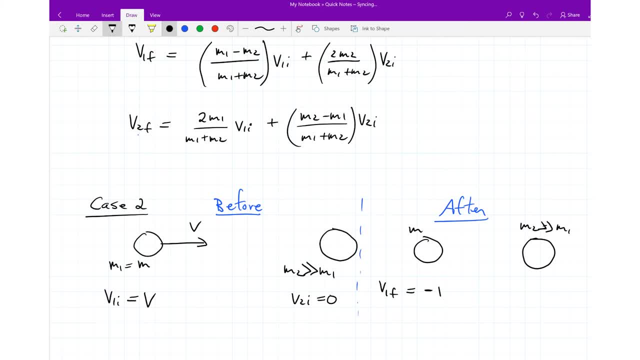 much, much bigger than m1.. So how is this going to be simplified? So we're going to be left with minus m2 over m2 for the first term and multiplied by the initial velocity of 1.. The second term ends up being 0, because 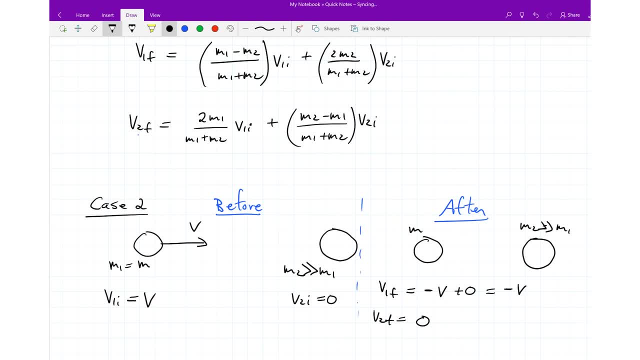 the initial velocity of object 2 is 0. You substitute all the variables in there. you get minus V for the final velocity of object 1 and you end up getting 0 for the final velocity of object 2, which is what you would expect. 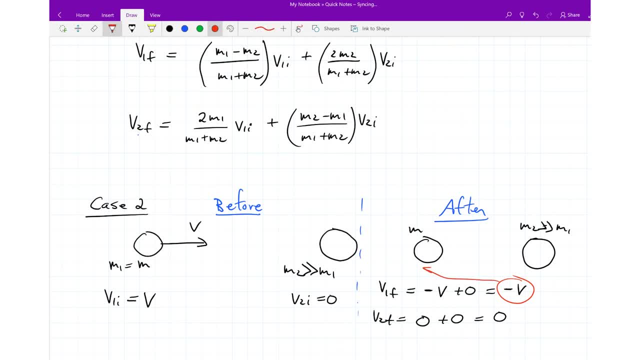 If you have a really, really massive ball, you don't expect it to move And you expect the object that's going to strike it simply to move backward. if it's a completely elastic collision, It simply bounces off and moves in the opposite direction. 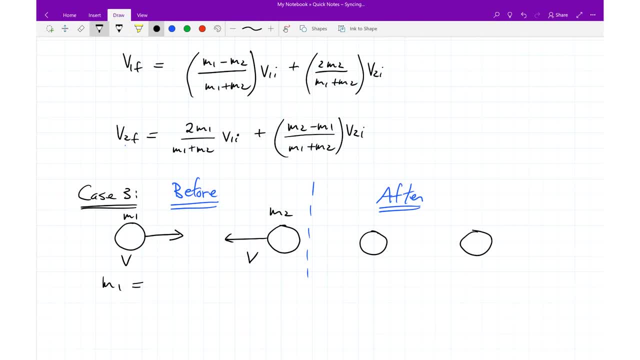 Alright, case 3 is a slight variation. now We have both objects moving toward each other at the same speed, but different directions. We're going to take the masses to be the same Again, since the masses are the same. this simplifies a lot of the terms and expressions above. 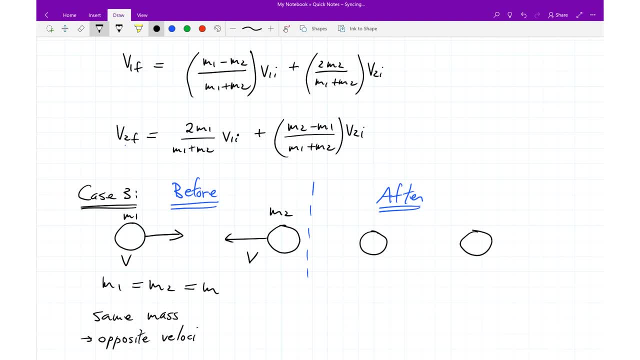 So they have the same mass but opposite velocities. Let's see what happens after the collision. So what do you think is going to happen? Again, if we first consider the final velocity of object 1, the top expression, the first term gives 0, because the masses are the same. The 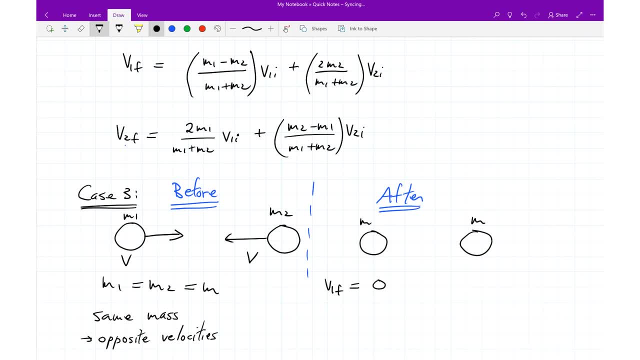 second term, on the other hand, that one was not going to cancel out. When you substitute in the masses m1- and m2 equals the m- into the top equation or the second term of the top equation, you end up getting 2m divided by 2m. 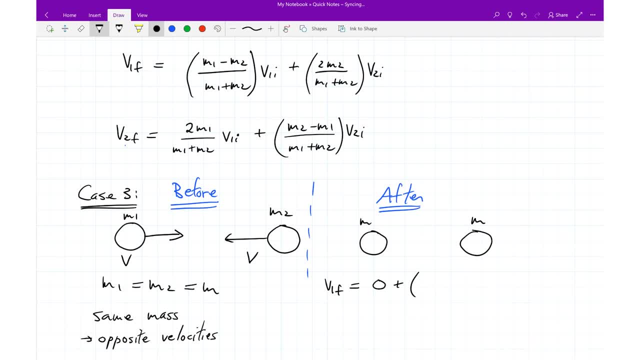 multiplied by the initial velocity of object 2, which is minus v, and the negative sign appears there because it's the direction. The direction is moving to the left and we're going to take that to be the negative direction. So, substituting everything in, you get minus v for the final velocity of object. 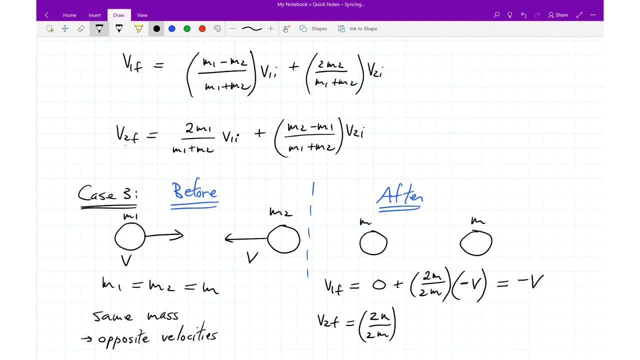 1. If you now look at final velocity of object 2 again, there's only one term that survives, Since the masses are the same. it simplifies and you're left with final velocity equals to v. So what does that mean for the cartoon? Well, it means. 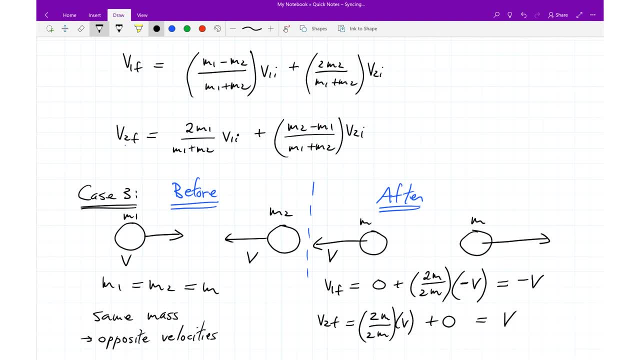 that object 1 is simply going to bounce off and move in the opposite direction and object 2 is going to bounce off. So this would be a case of just billiard balls colliding And then bouncing off each other. Again, the negative signs in these expressions. 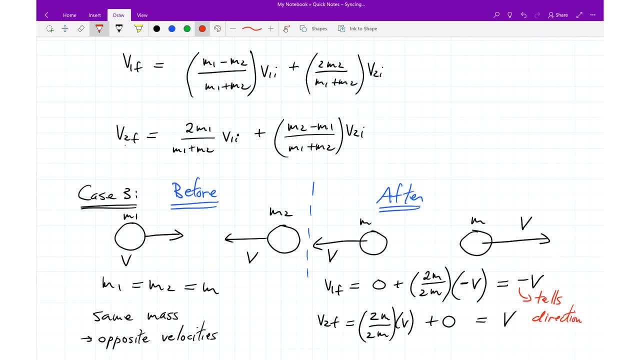 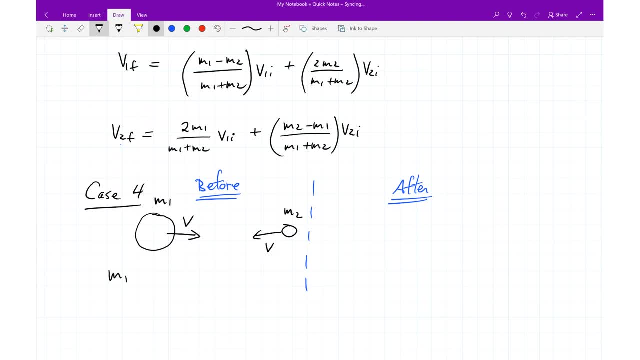 simply tell you something about the direction of the velocity. Kind of a nice example. Alright, in the final case I want to take again both objects coming toward each other, except this case, I'm going to take the mass 1 to be much, much bigger than. 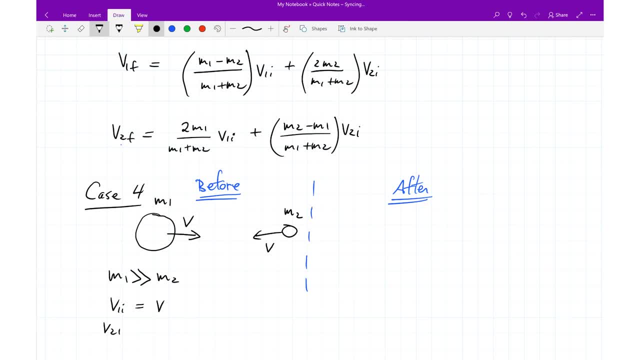 object 2.. They're both going to have the same speed, their velocities in the opposite direction. So I put a negative sign for the initial velocity of object 2.. Again, we want to see what's going to happen after the collision. Again, I always use a. 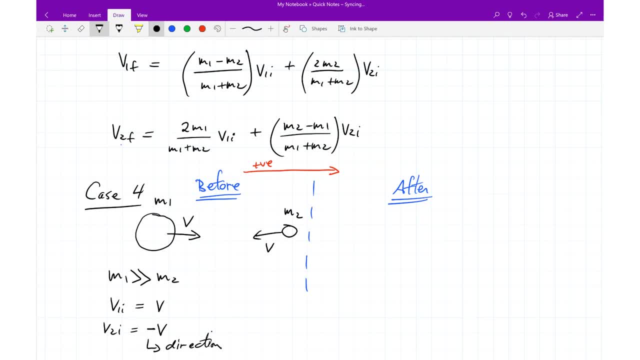 coordinate system where anything pointing to the right, any velocity pointing to the right, is a positive velocity when I substitute in the top two equations. So what happens after? Well, I have m1 and m2 again Again, when you take the limit you can or when you substitute in the above equation. 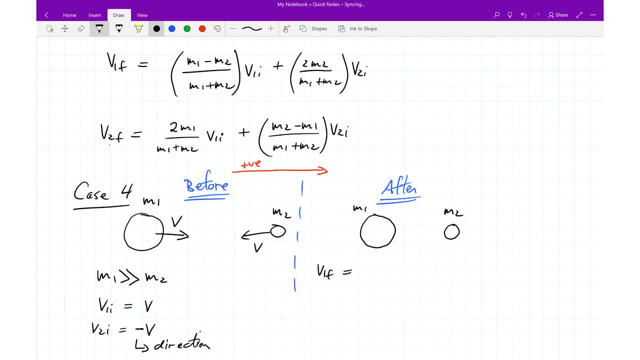 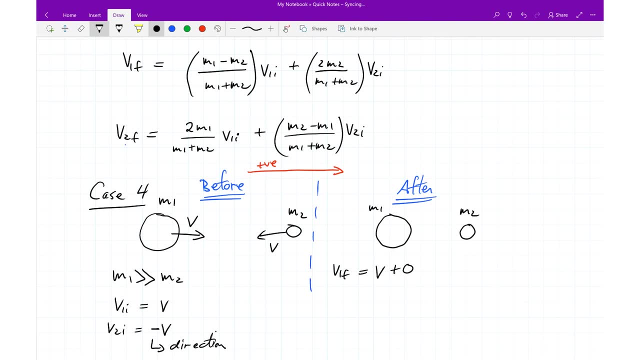 I don't have to consider the effects of m2 because m1 is so much bigger and it's the dominant term. So for the first term I simply get V Masses cancel out, and the second term I'm going to be dividing by m1.. Which is very, very big compared to m2. 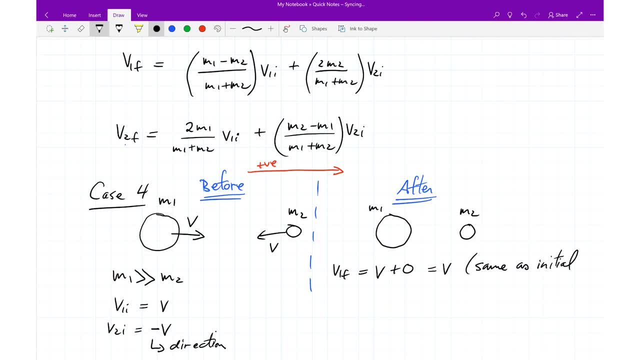 So it's 0. so you notice that object 1 Is simply going to keep going. it's as though m2 is not even there. It doesn't slow down at all. its final velocity is exactly what its initial velocity was. What about object 2, on the other hand? 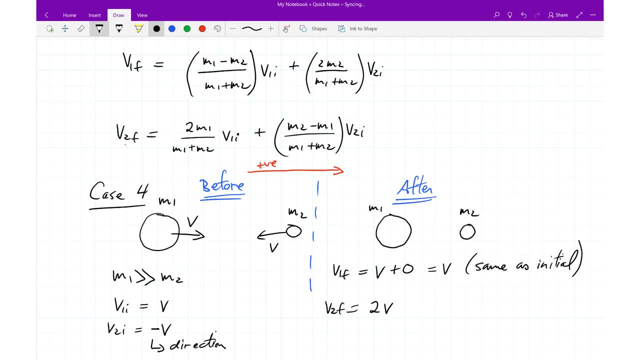 again. we substitute the velocities and you take the limit when m1 is much, much bigger than m2. the first term simplifies to 2v and The second term on the end. you got to be a little bit more careful. You're going to be left with minus m1 over m1. 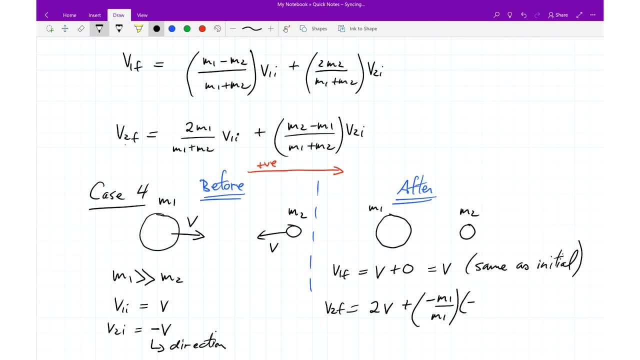 multiplied by minus V, And again minus, because that tells you something about the direction of the velocity of object 2 initially. Combine both of those, you get 3v. So put that on the diagram here: object 1 is moving at velocity V after the collision and object 2 is moving at 3v. 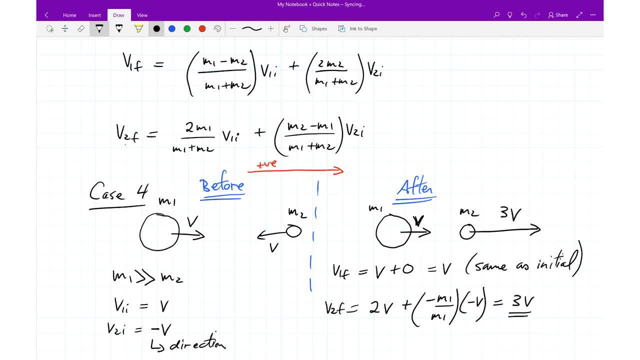 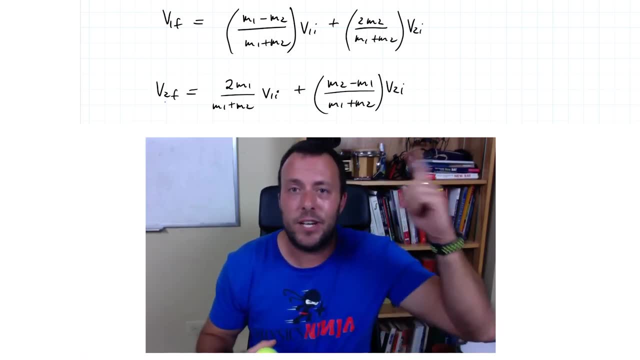 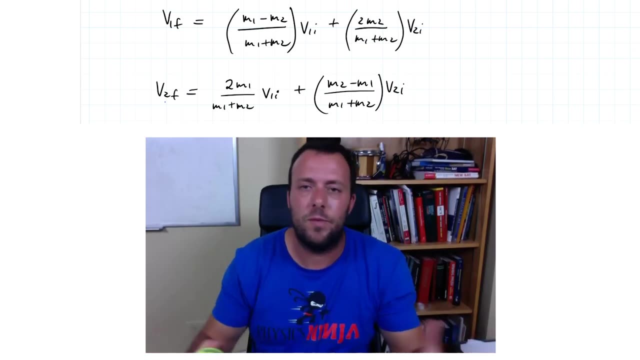 after the collision. Well, thanks for watching the video. so today I looked at one-dimensional collisions. we derived the expressions above And I looked at four different collisions involving two different masses. They could be the same, may be moving in different directions, Sometimes one objects not moving and I looked at how you apply those equations to calculate the final velocities of both objects. 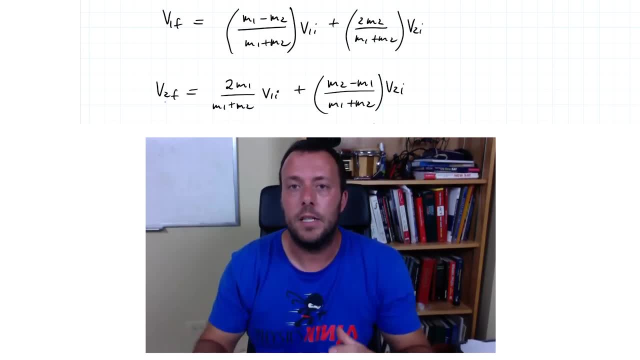 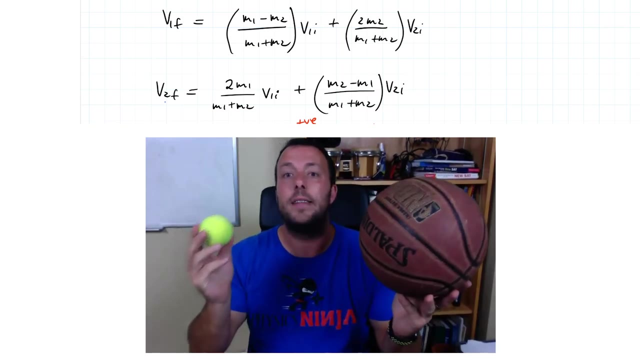 The case number four was kind of an interesting case. It's where object 1- the mass of object 1, was much, much bigger than the mass of object 2. In another video I'm going to actually apply that equation and look at the collision between a basketball and a tennis ball and see what happens. 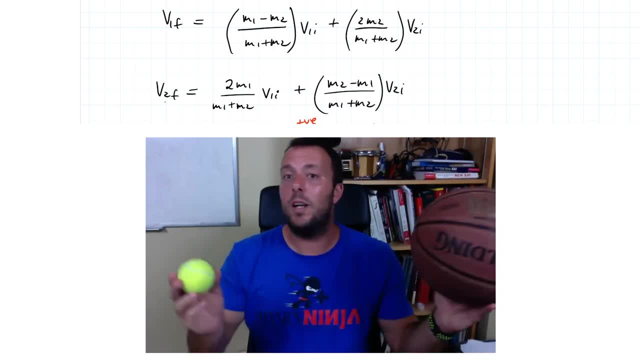 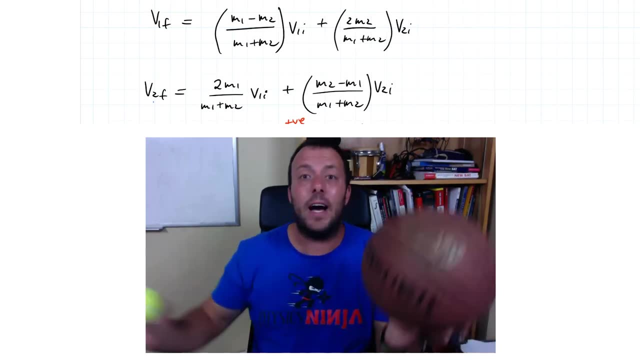 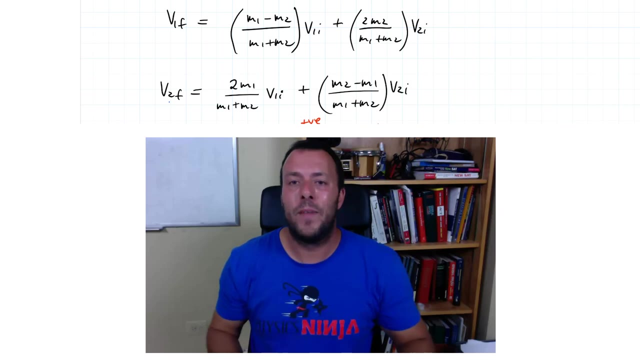 We just saw from case number four that object 1 continues as though object 2 is not even there, And object 2 had a velocity three times the velocity of object 1. So let's apply that to the tennis ball and the basketball problem. So have a look at that video. 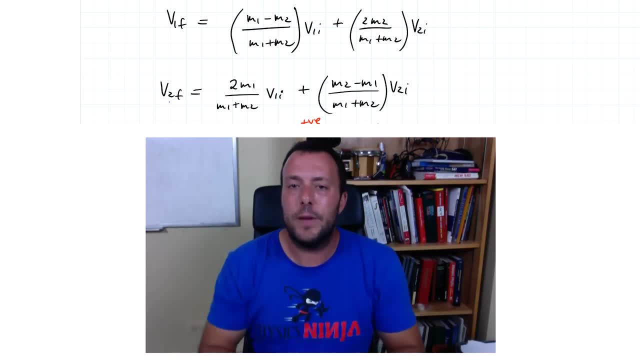 Tell me what you think. Consider subscribing to my channel. if you have any questions about any of the videos, I do, don't hesitate to leave a comment or send me an email. Thanks for watching.